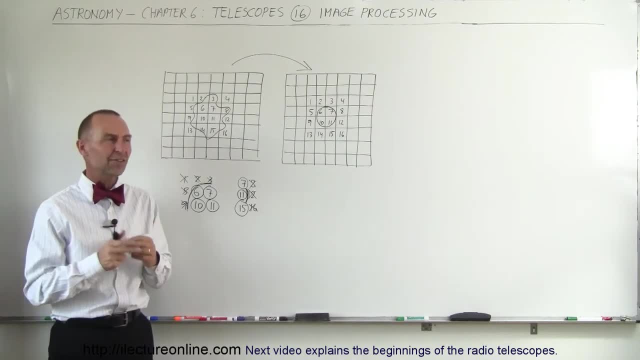 do image processing using our very powerful computers. How does that work? Well, now that we use CCDs and pixels in our image capturing, so that each pixel actually captures a certain amount of light from the image that we're trying to take, we can take something that looks blurry like this and make it into 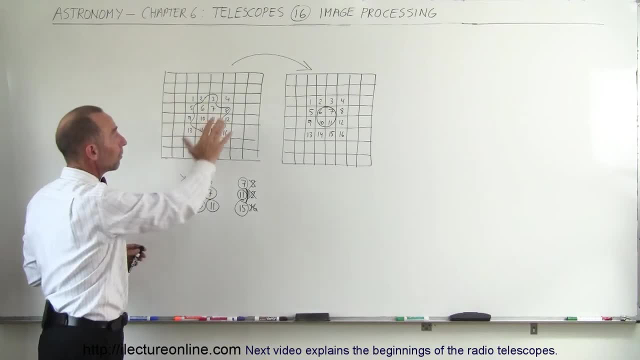 something that looks very sharp. and how do we do that? Well, let's say that we number our pixels, and here's just a small example. and let's say we take pixel number six, that's our central pixel. we're going to look at all the pixels around number six and when we do that, we notice that pixel number six has 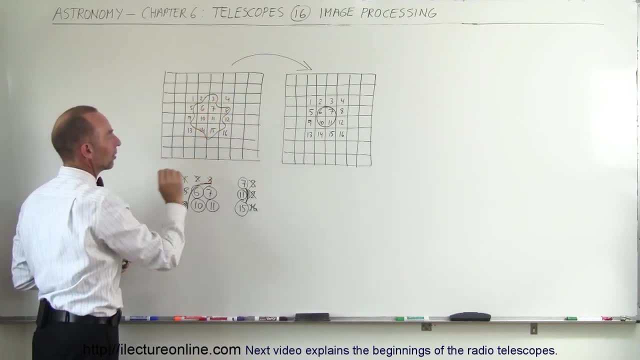 a full intensity image. pixel number seven has a nearly full intensity image, so does ten, and so there's eleven. so they pass the threshold of receiving enough light to say, yes, the information on those pixels is relevant. but then if we look at number three, two, one, five and nine on the outside, there you can see. 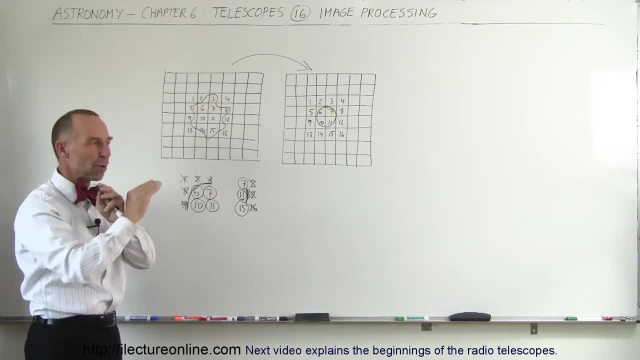 that they only have a partial influx of energy and therefore we would then reject that as saying those are not relevant to the picture. we then end up rejecting it, and so we integrate all this information into pixel number six and say pixel number six has enough information, has enough light energy. 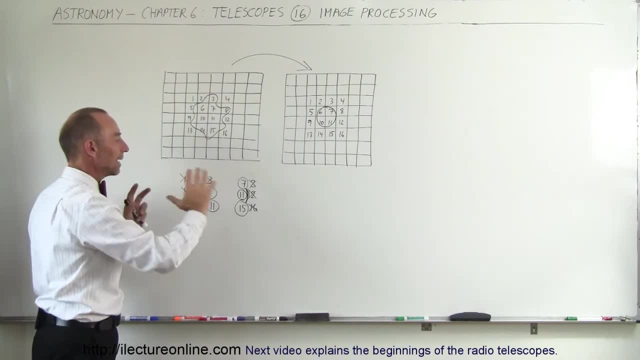 there has enough photons collected to want a lot. that is part of the image. So that's what we're going to do and that's what we're going to do next. The final image also. seven, ten and eleven are our full pixel images. so we 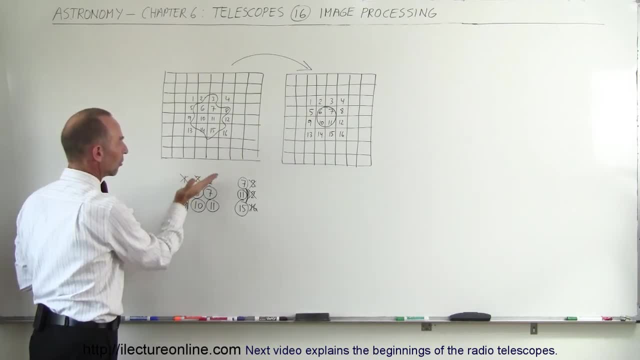 know that the image is relevant in that direction and irrelevant in this direction, so we simply subtract that from the image and we end up getting something that looks like: this is relevant to the picture and this is not, which would then turn into something that looks like this: where six, seven, 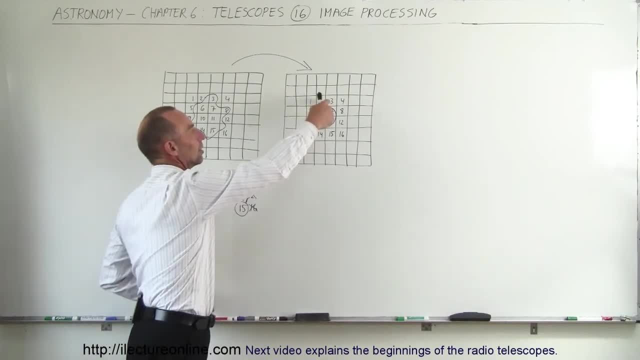 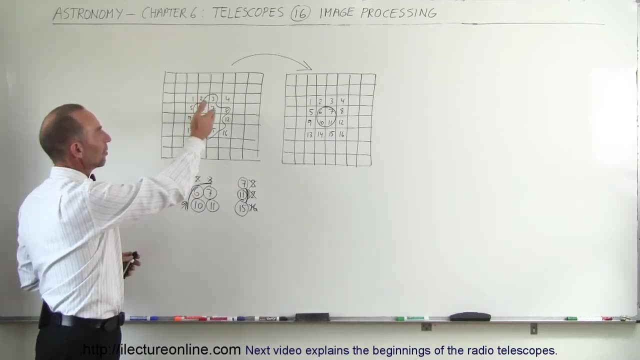 eleven, ten are all relevant, but the pixels underneath there are not, and so we discard that information to make it into a sharper image. For example, let's say that number eleven is our central pixel. so we take a look at number eleven, seven and fifteen have irrelevant. 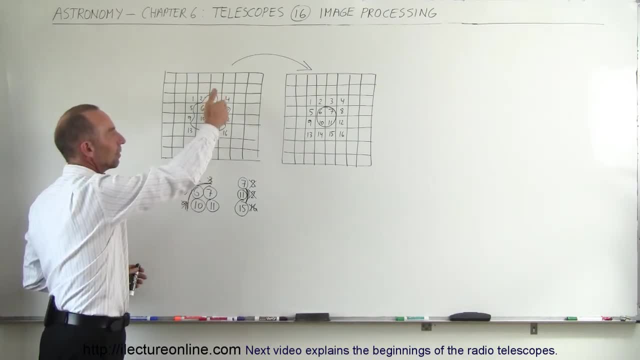 information. so we keep that. but eight, twelve and sixteen, they don't have enough light information there, we end up discarding that information. so for pixel number eleven, we integrate all the information in. We only deem it relevant on this side, none on that side. so you can see that seven-eleven would be relevant and the rest not, and that. 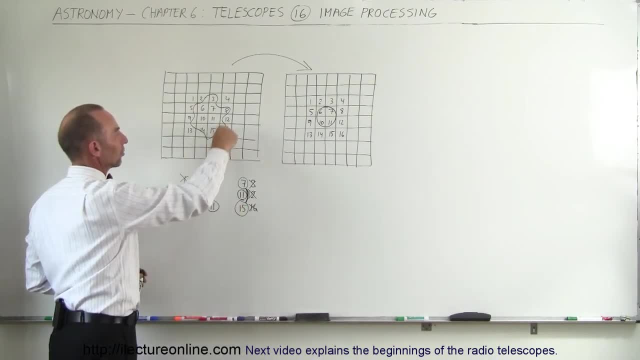 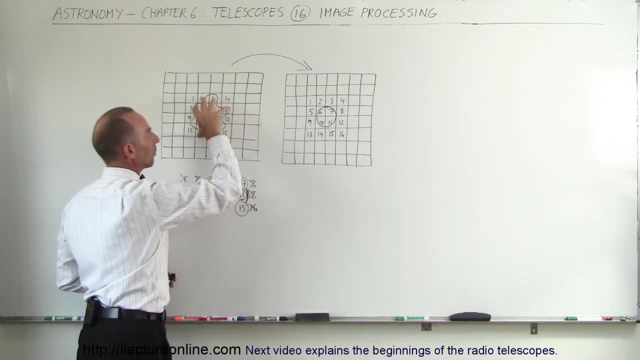 gets discarded. We would do the same thing at number fifteen. notice that the pixels around there are not relevant, so 15 would only have partial relevance to may or may not be included in the picture, and so, in that respect, by doing this over and over again, 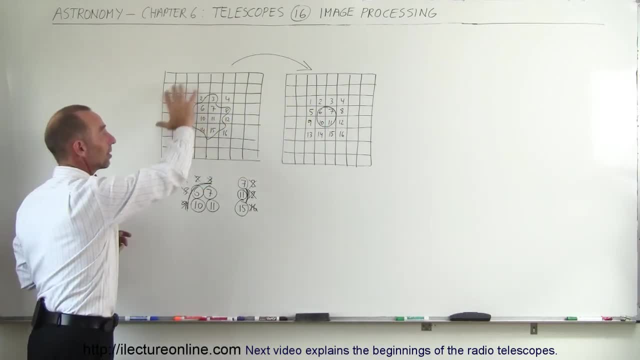 for every single picture on the, on the, on the, for every single pixel on the image. we can take something that looks blurry and then reprocess it in something that looks sharp and more defined to get the information that we look for, and we do that a lot with our pictures that we take. 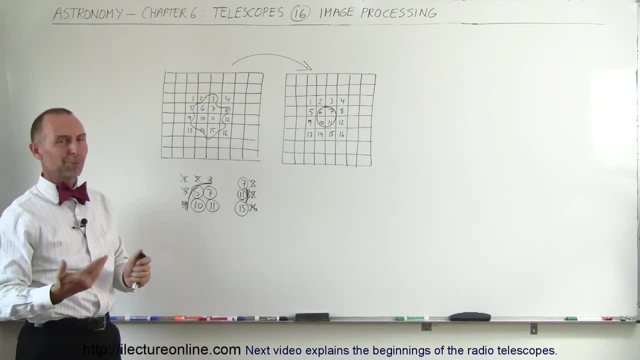 computers can do all the work. we don't have to do any of it except write the computer programs, of course, and so that's another technique for us to take those blurry images, especially because of the atmospheric interference, and make them into something sharp and meaningful. it's amazing what. 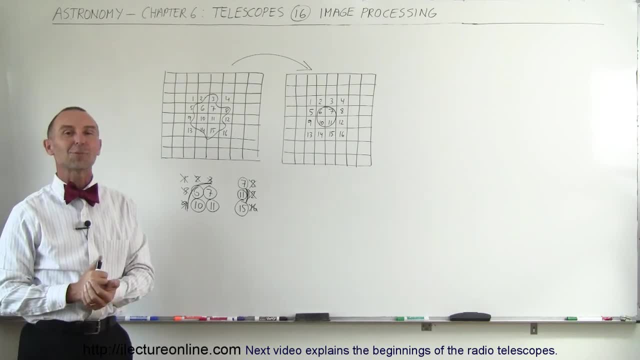 computers can do for us these days for astronomy. that's what we call image processing. 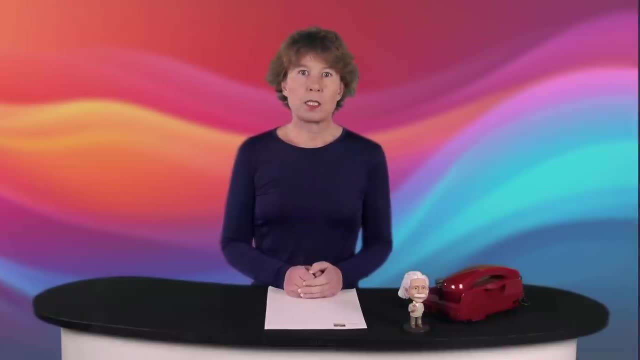 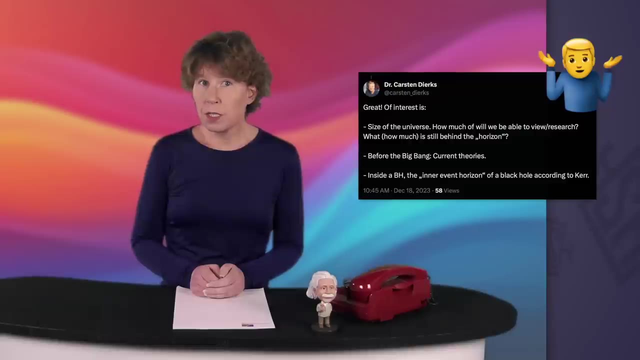 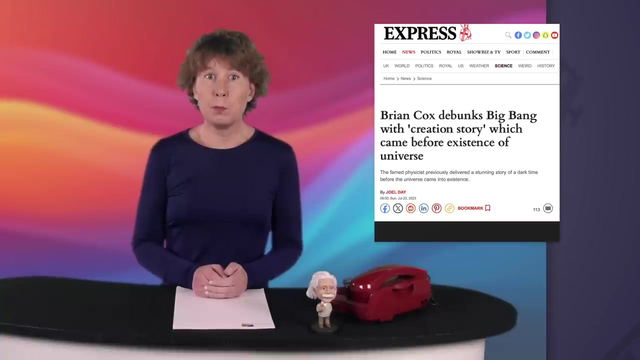 What happened before the Big Bang? I got this question on Twitter and thought: well, the answer is that we don't know. Now, I'm quite fond of short videos, but that's a little too short even for my taste. Then I saw that Brian Cox has supposedly debunked. 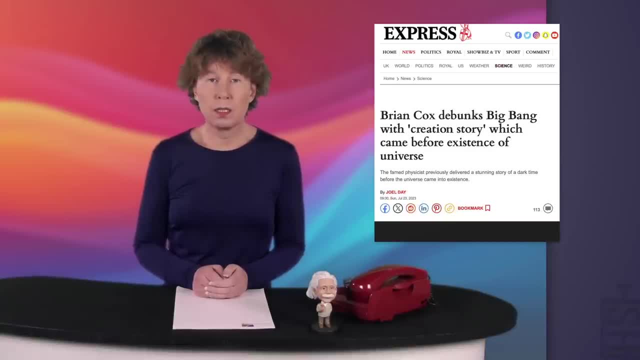 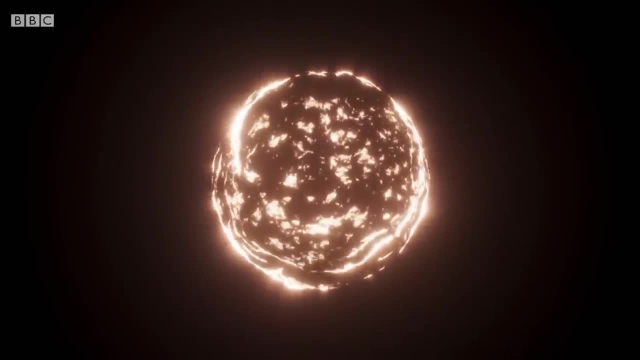 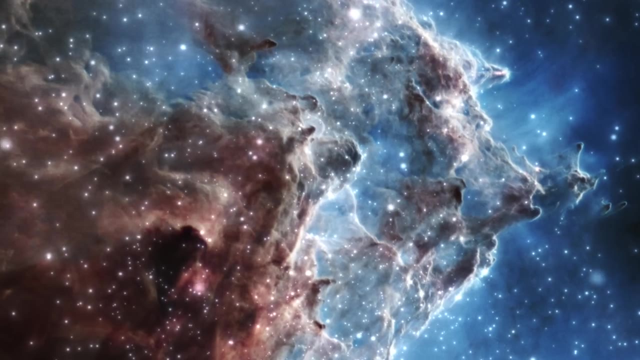 the Big Bang with a creation story and I thought he did what? Then I watched the clip that's narrated by Brian Cox and I think I know what happened there. Let me explain What happened. Observations tell us that the universe expands. If we use those observations and take the